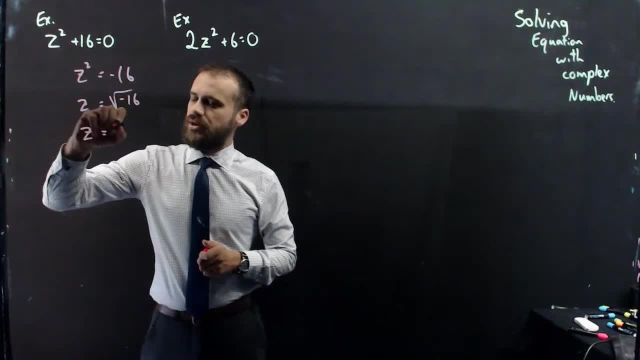 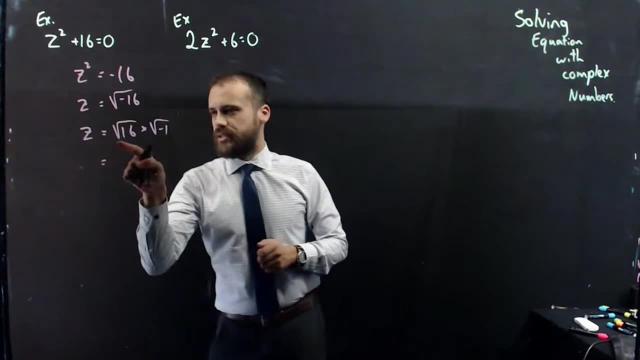 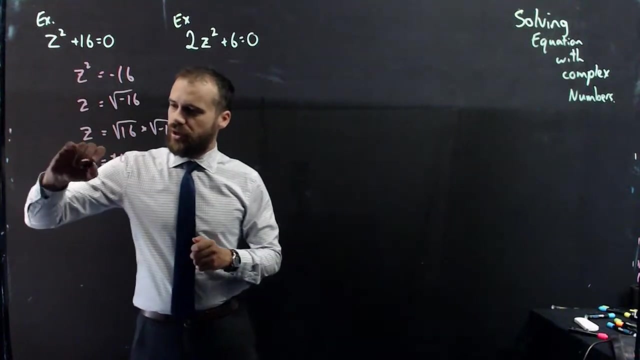 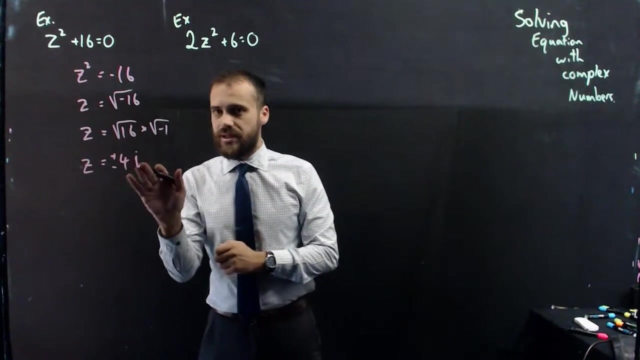 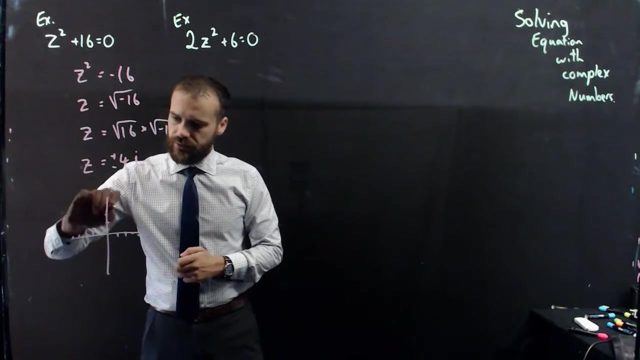 square root of negative 16, so z equals the square root of 16 times negative 1, that's plus or minus 4, and that is i. We have two solutions, both purely imaginary: positive 4i and negative 4i. I can draw them on an R-game diagram if I want to. There at 4i. 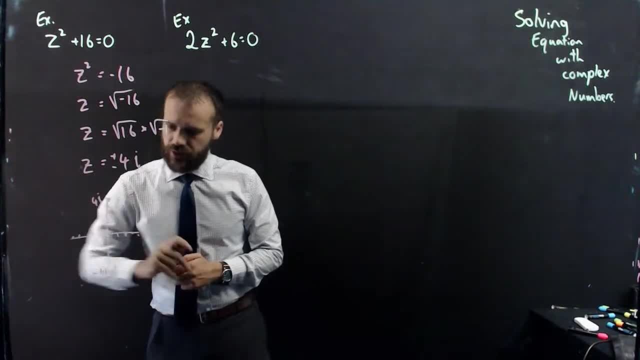 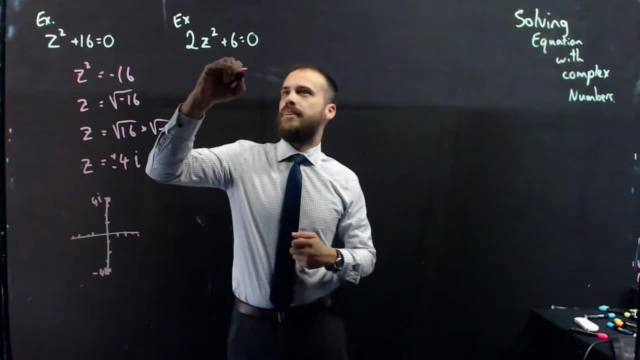 and 1,, 2,, 3, 4, at negative 4i. There are our two solutions. It's 2z squared plus 16 equals 0.. Oh, let's jump straight into this one. So 2z squared. 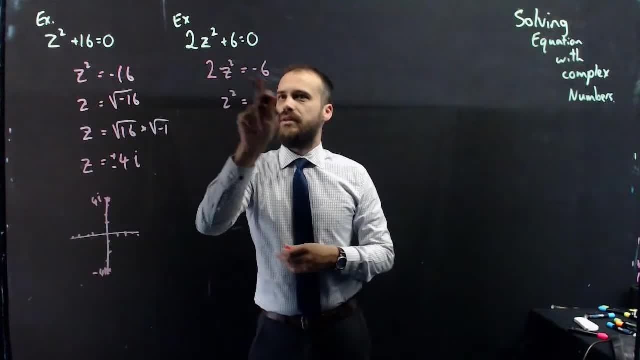 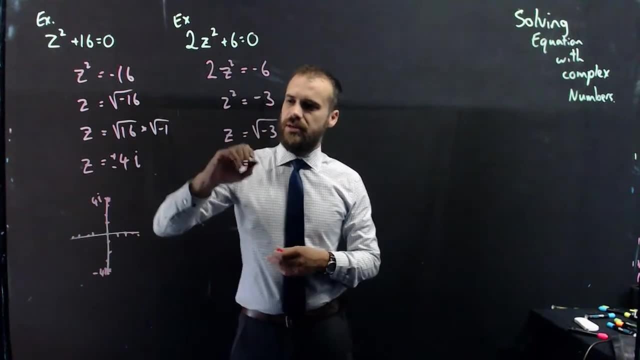 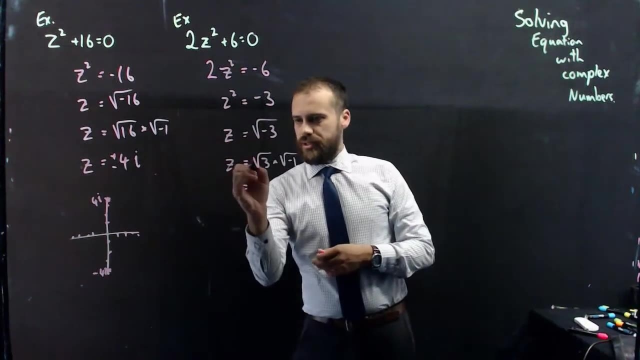 negative 6, z squared. negative 6 divided by 2 is negative 3,. z equals the square root of negative 3, which means that z equals root 3 times root. negative 1, plus or minus. let's put the plus or minus a step earlier, I think. 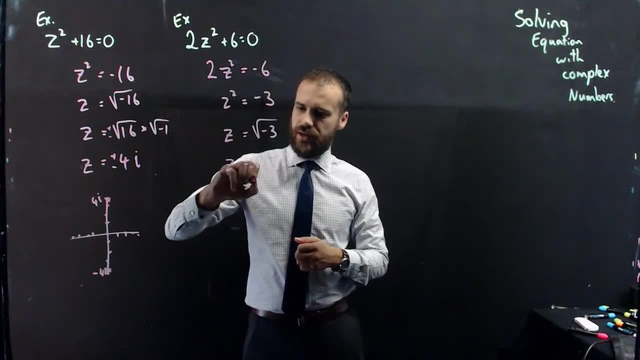 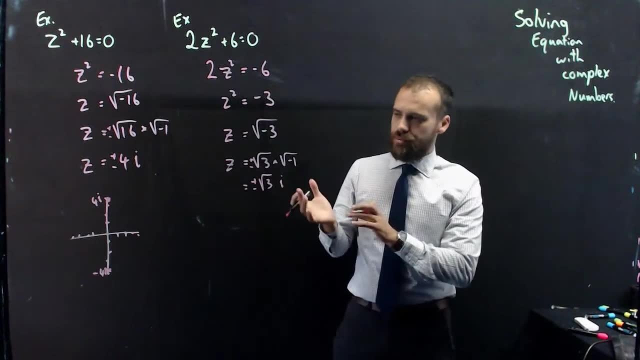 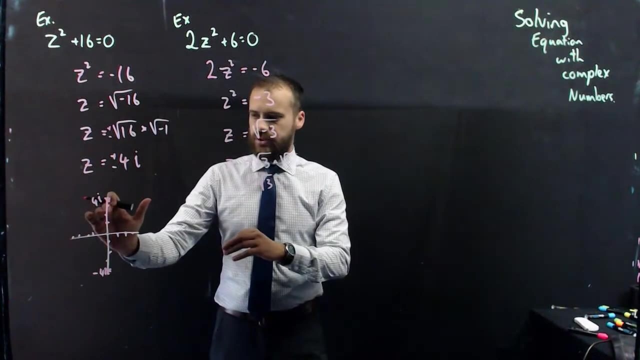 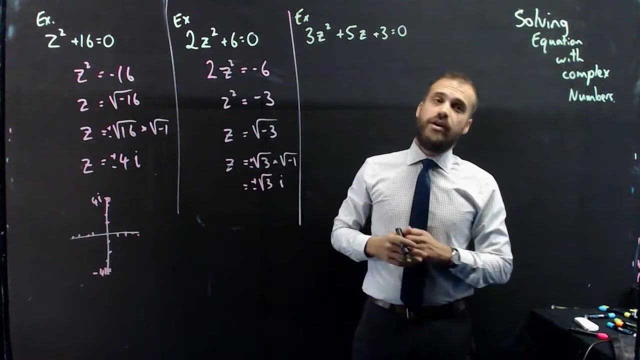 Okay, so what we have here now is plus or minus root 3i And again purely imaginary. we can put it on our complex number plane, sorry, on our R-game diagram: positive root 3i, negative root 3i. So a little more work to do. in this example, 3z squared plus 5z. 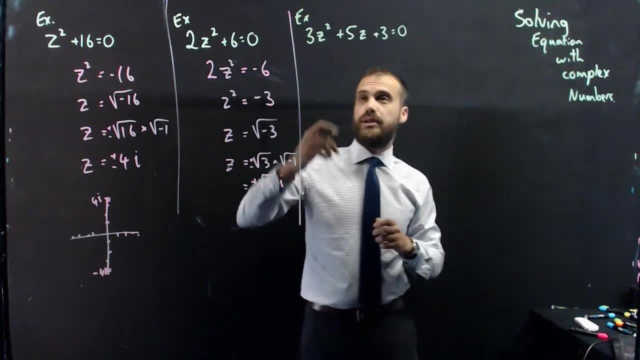 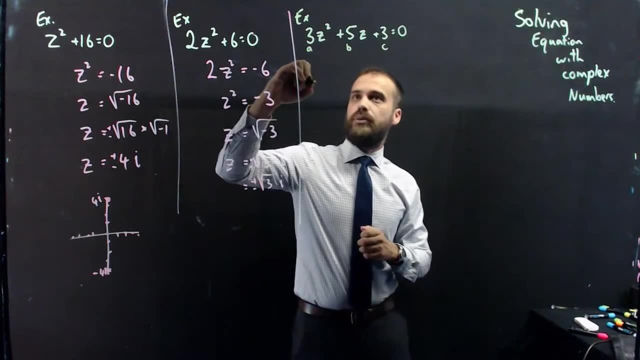 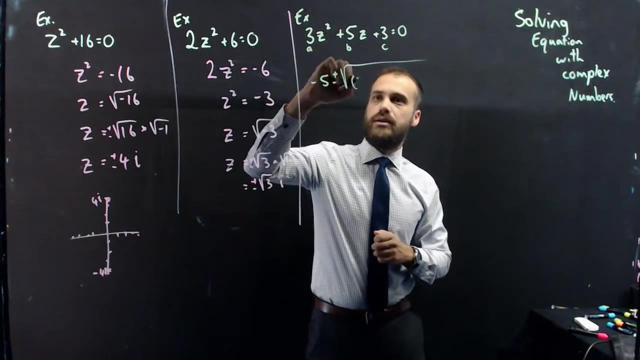 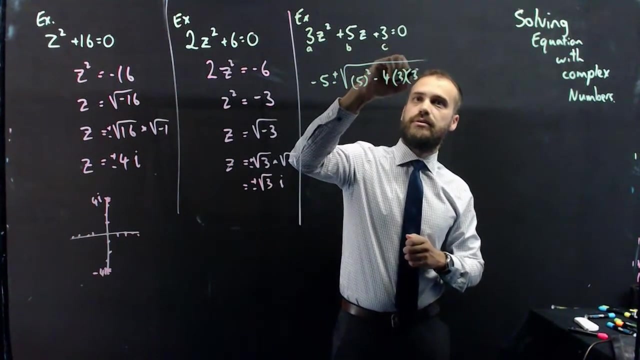 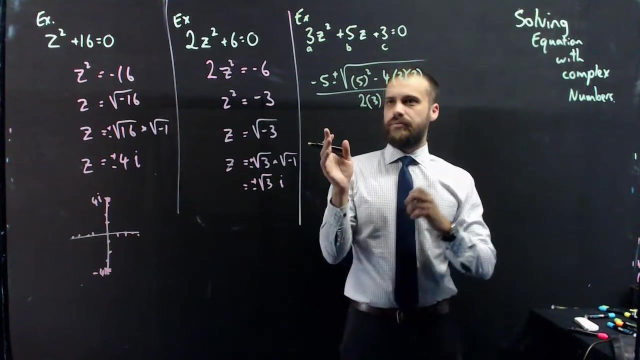 plus 3 equals 0.. I'm just going to use my quadratic formula here. This is our a value, this is our b value and this is our c value. We have negative b, plus or minus the square root of b squared minus 4ac, all over 2, 3.. All right and from. 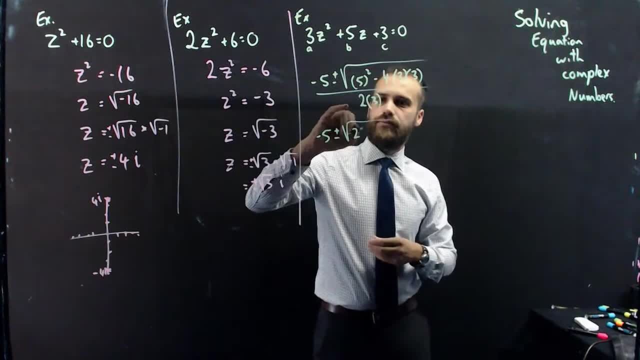 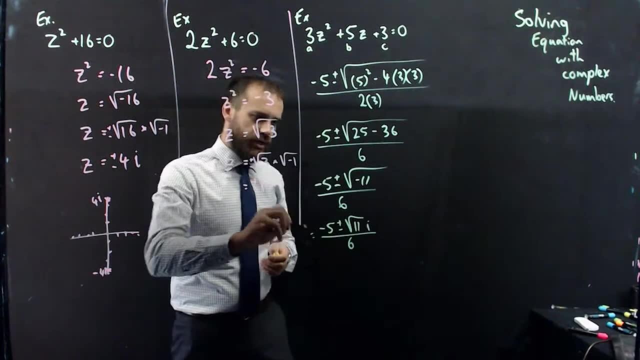 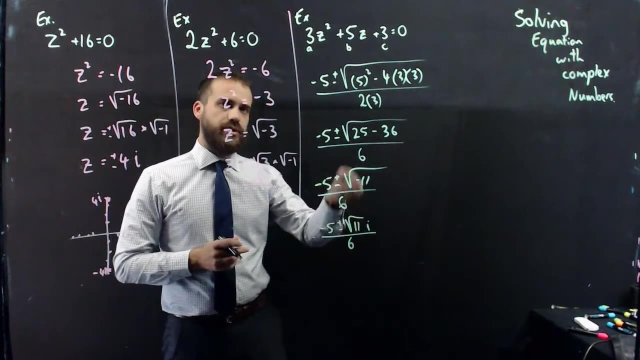 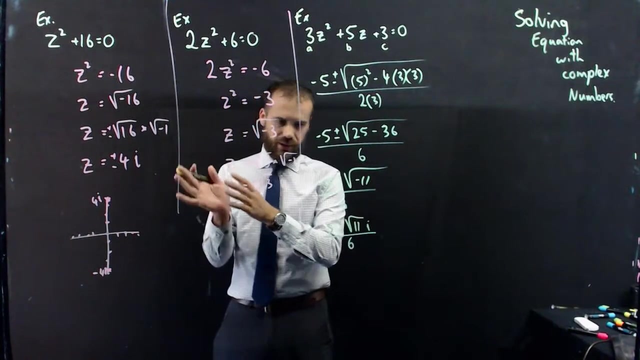 there we can just sort of do some numbers. Okay, we can stop there. We've got two solutions here: negative 5 plus root 11i over 6, and negative 5 minus root 11i over 6.. So a little more complicated than these two, but same.